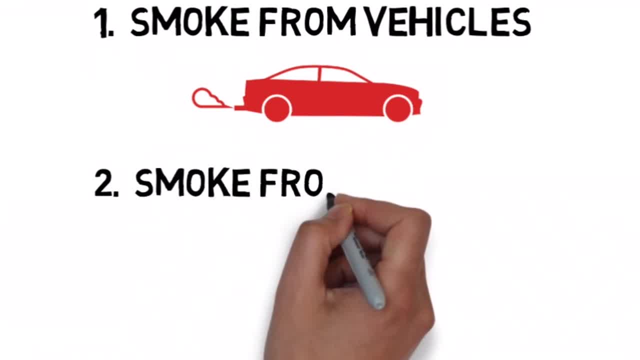 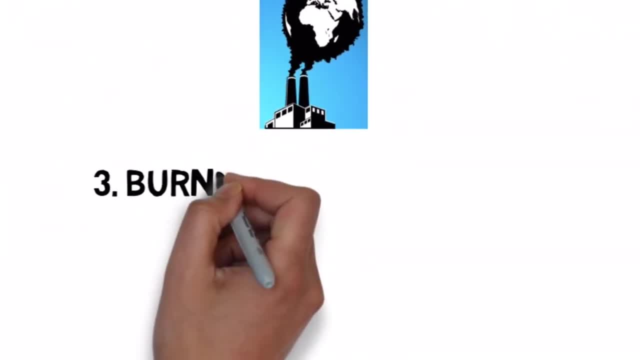 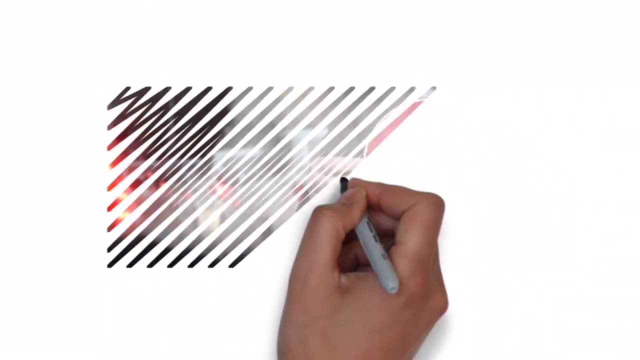 number one. the smoke emitted from vehicles, the smoke released from factories burning of fossil fuels like coal and petroleum: They all are reasons or causes for air pollution. All these activities add toxic gases such as carbon monoxide, nitrogen dioxide, carbon dioxide, to the air that 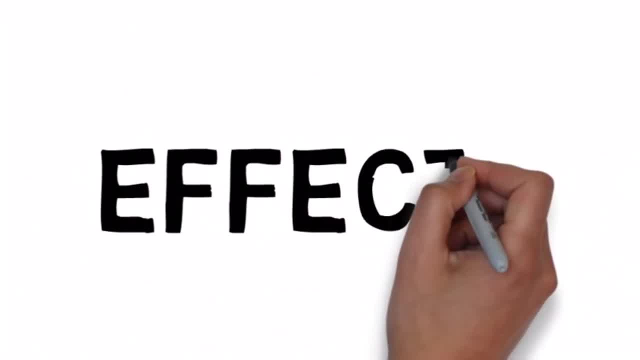 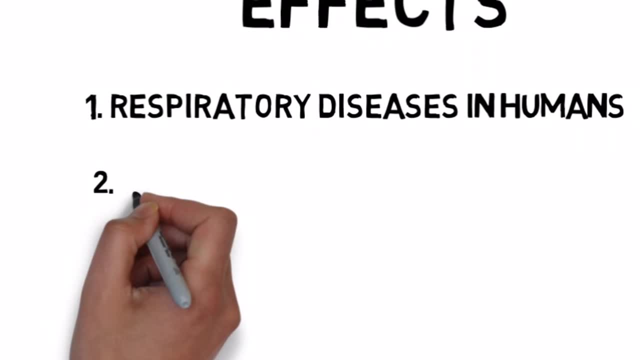 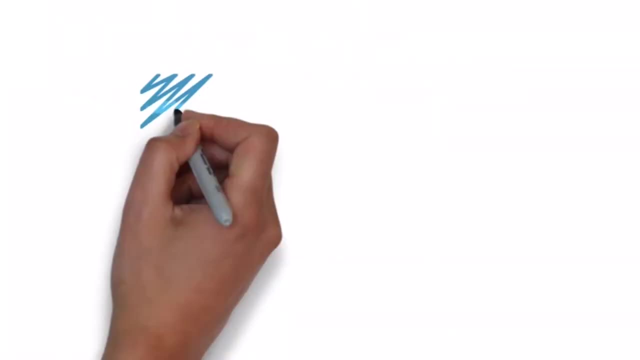 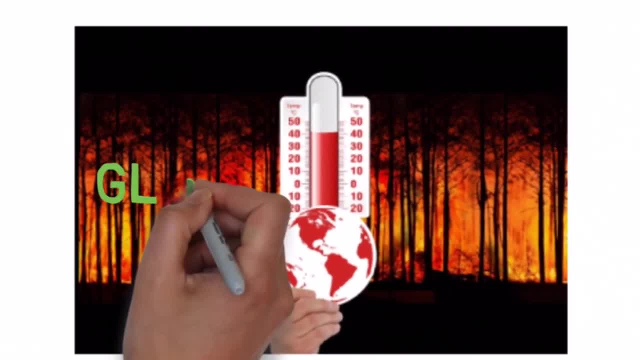 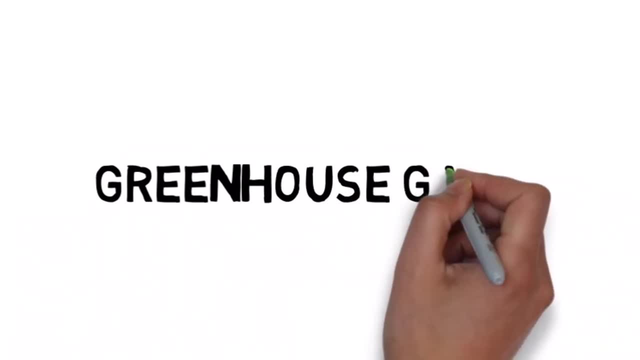 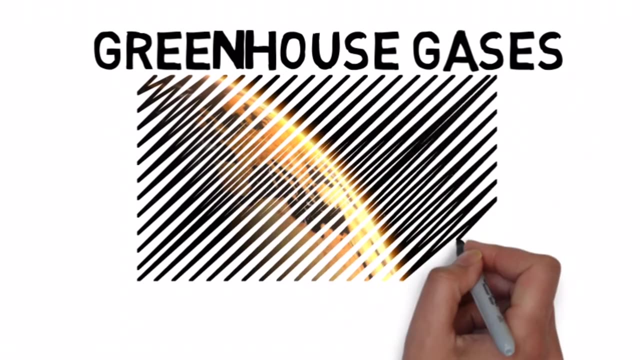 harming us, but also our planet, by way of global warming. We have heard or read in many places that air pollution is leading to an increase in greenhouse gases. Now, what is this? greenhouse gas or greenhouse effect? Greenhouse gases actually include gases like carbon dioxide. 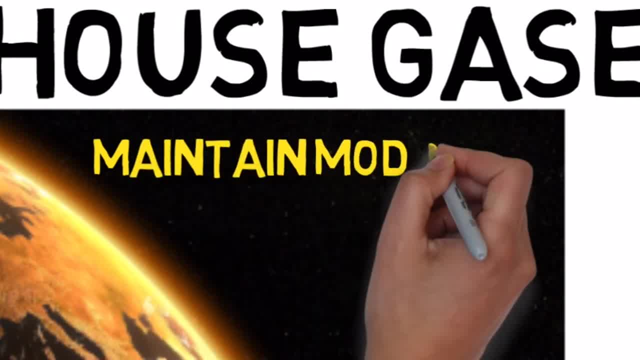 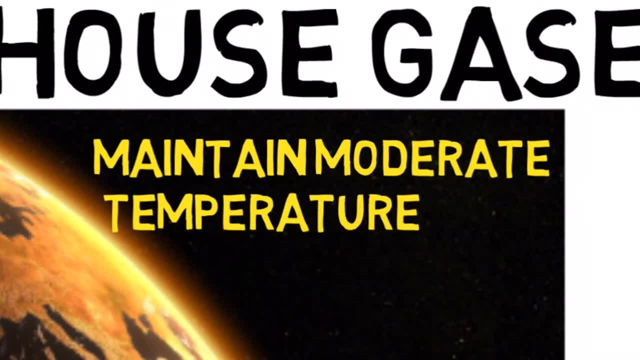 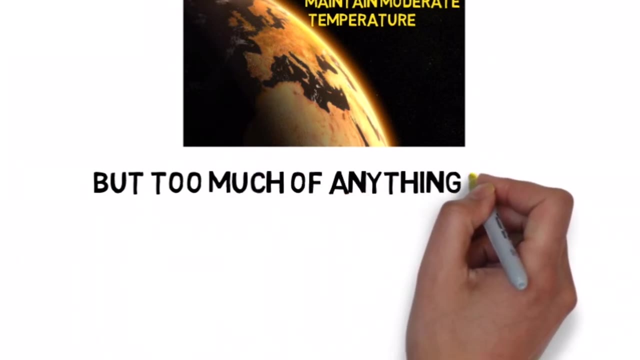 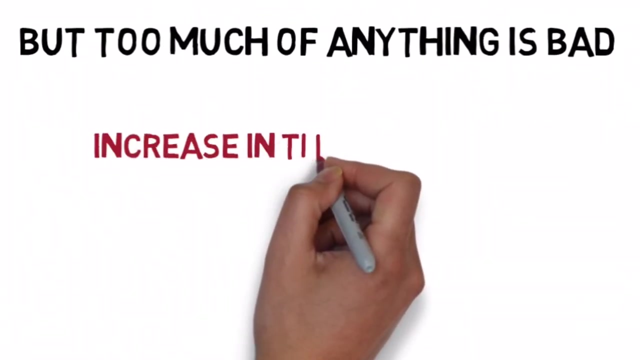 and methane, and these gases actually prevent our earth from freezing cold temperatures. They trap some amount of heat from the sun and prevent it from escaping our earth, thereby maintaining a moderately warm environment, which is good enough for living things to survive. However, the greenhouse effect can cause more heat to get trapped in the earth, and when more heat is trapped, 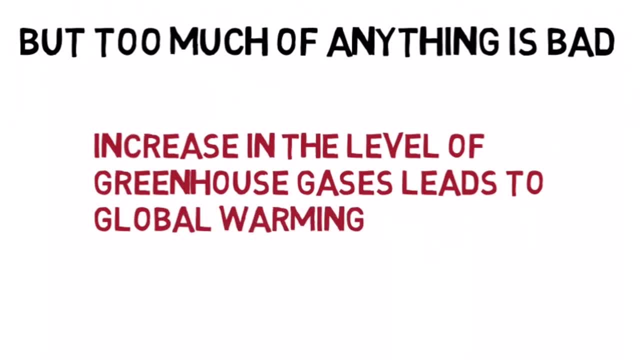 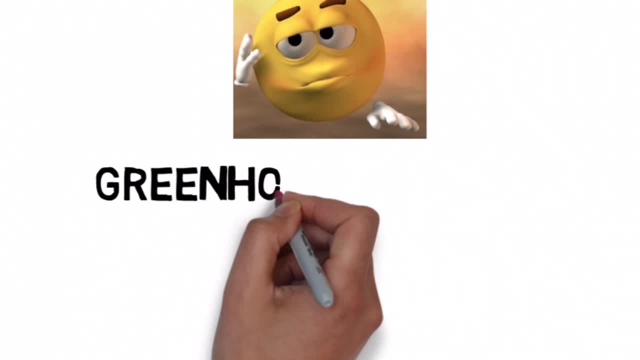 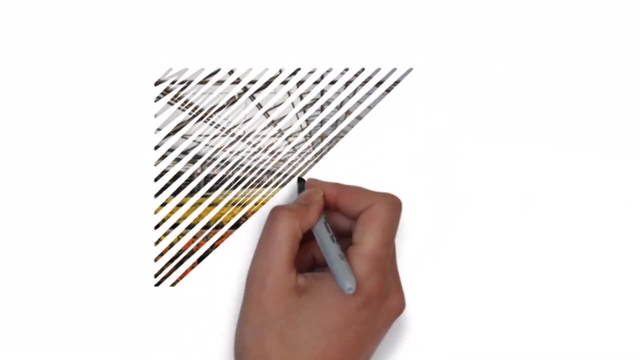 the result in increasing average temperature of the earth, which is called global warming. Now, haven't you ever wondered why is it called greenhouse effect? A greenhouse is a glass house used to keep and grow plants that require warm temperatures. The glass roof is opened. 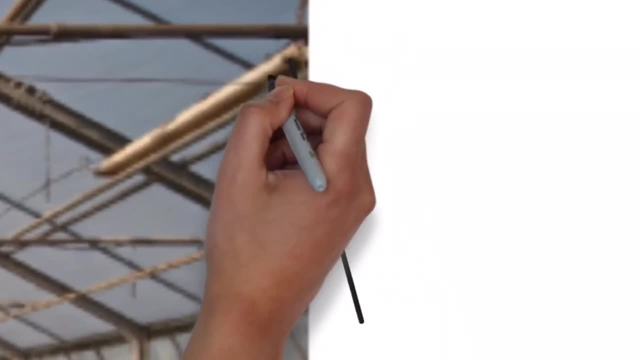 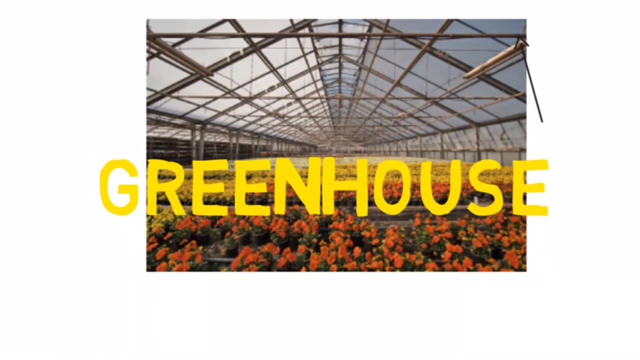 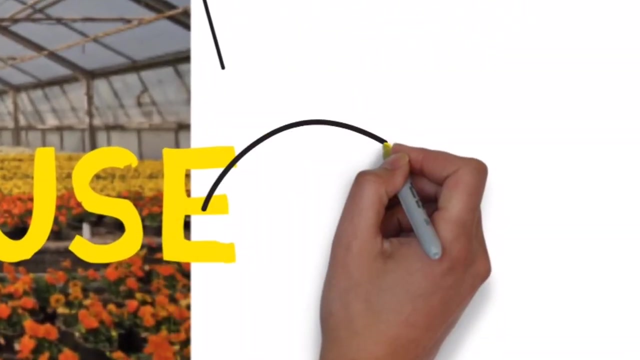 in the morning to let in the heat and sunlight from the sun, and closed before sunset. The glass acts as an insulator and does not let the heat escape, thereby keeping the nursery warm. The same function is carried out by these gases, which are called greenhouse gases.